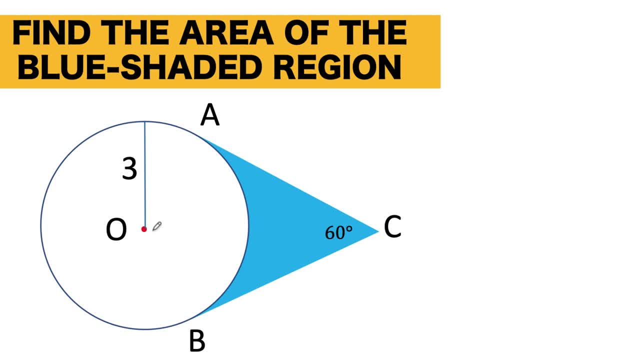 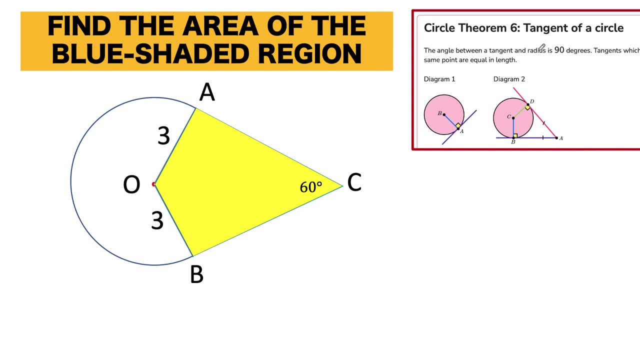 and since radii of the same circle are the same, then segment OA must also be three units. The same thing with segment OB. Notice that we have here a quadrilateral AOBC. Let's recall some properties of a circle From the tangent of a circle theorem. 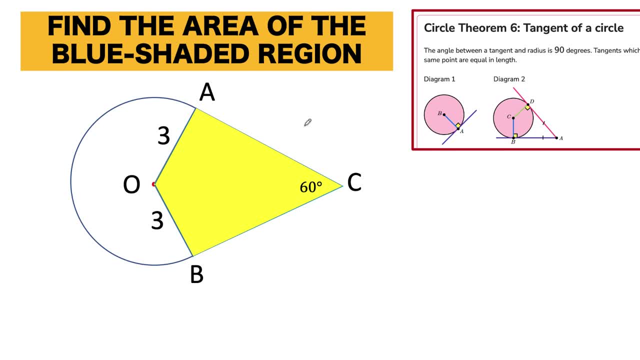 the angle between a tangent and radius is 90 degrees, meaning the angle here is a right angle. the same thing with angle OBC, Both of them measured 90 degrees, Also from the same tangent of a circle theorem, tangents which meet at the same point. we have here two tangents, AC and BC. 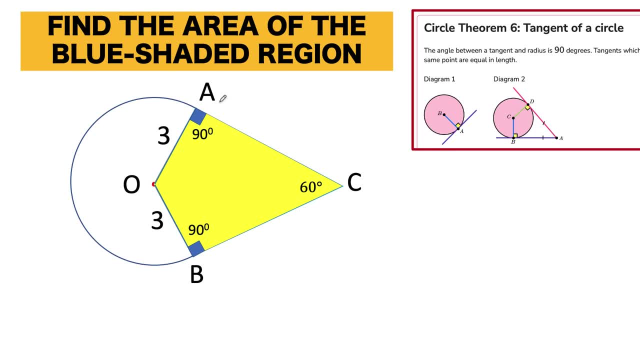 that meet at point C are equal in length. So that means segment AC is congruent to segment BC. Now, since we have here a quadrilateral AOBC, we have to find what is the area of the circle. Let's look at a quadrilateral and we know the measures of the three angles. then we can compute for the. 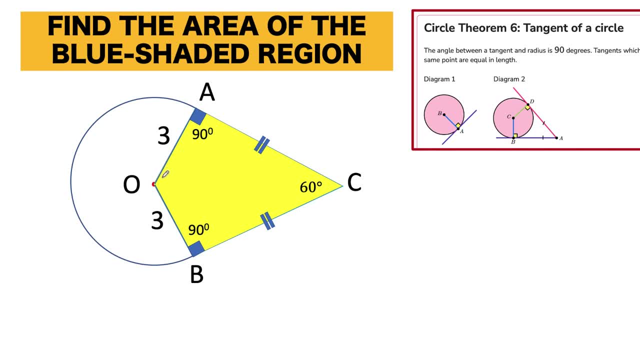 measure of this remaining angle. So if we let x be the measure of this central angle, then x plus the sum of these three angles equals 360 degrees. That is because the sum of the interior angles of a quadrilateral is 360 degrees. So solving now for x, we have: x equals 120 degrees. Let's remove this. 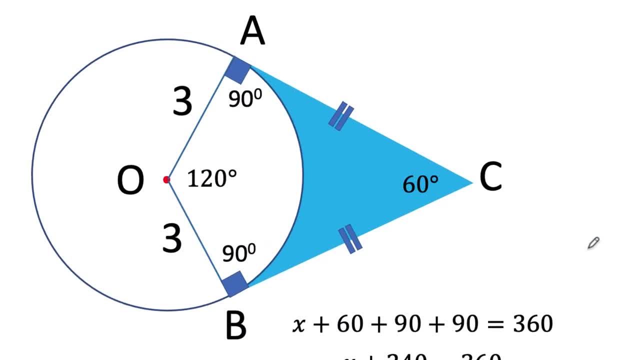 quadrilateral. So we want to find the area of this blue triangle. We want to find the area of this blue shaded region. Now let's construct these two triangles. We have this red triangle and this yellow triangle. What can we say about these two triangles? Notice that this side is three units. 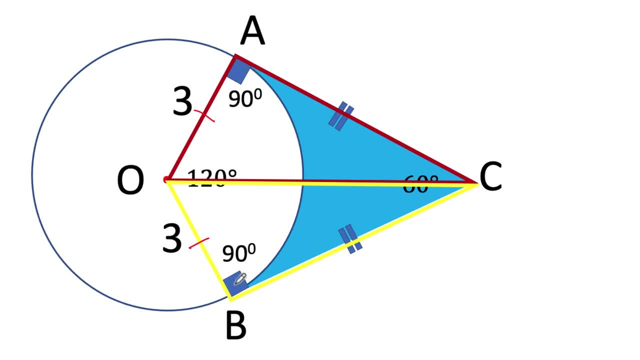 the same thing here three units. We have here a 90 degree angle and we have here two congruent sides. So from side-angle-side theorem these two triangles, this red triangle and this yellow triangle, are congruent, So their corresponding parts are also the same. That means these two. 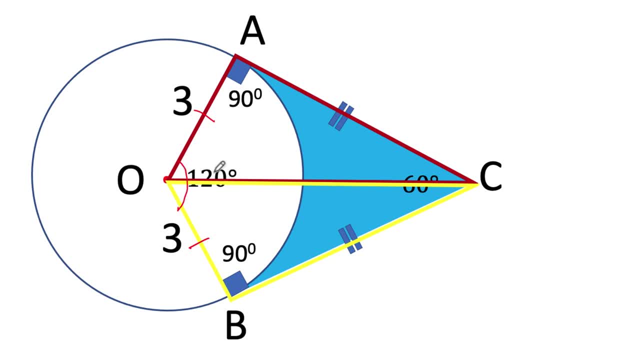 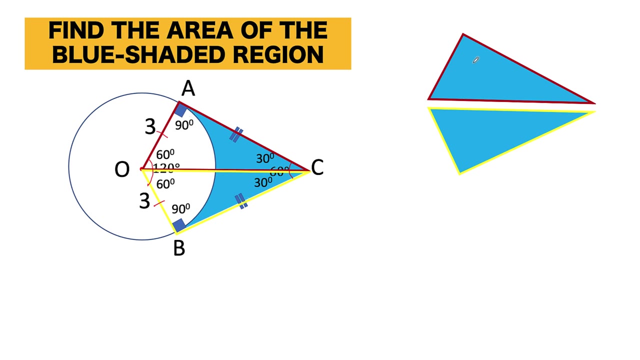 angles here, which is 120 degrees, must be divided by two to get 60 and 60 degrees for these corresponding angles. The same thing with the 60 degree angle. we split that into 30 and 30 degrees respectively. Now, in order to find the area of this blue shaded region, we can get the sum of 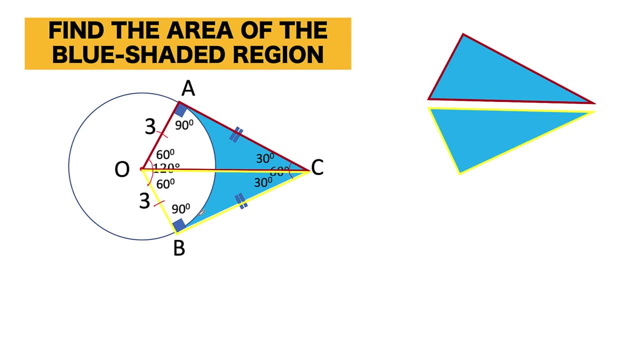 the areas of these two triangles minus the area of this sector, And let's detach that sector as well. What are their dimensions? We have a 30, 60, 90 triangle. This is also a 30, 60, 90 triangle and the measure of this side is equal to the radius. So we have 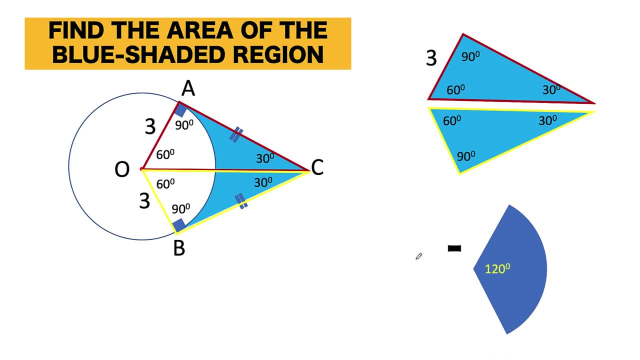 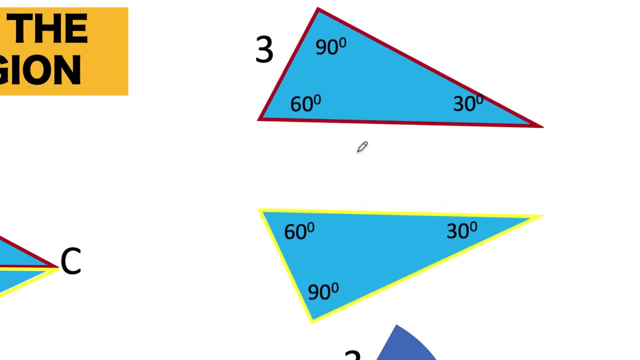 three units here And for this sector the central angle is 120 degrees and the radius is also three units. So let's find the area of these two triangles. If you can find the area of one triangle, just multiply it by two to get the sum of the areas of these two triangles and we are. 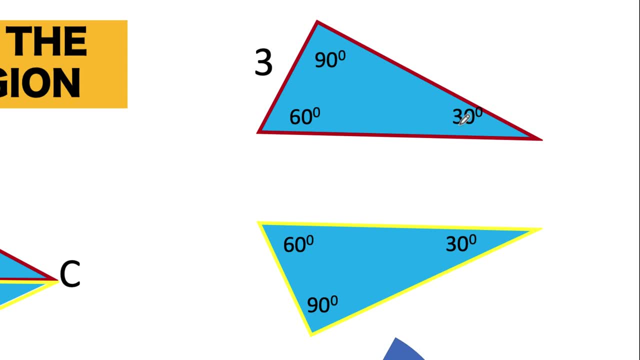 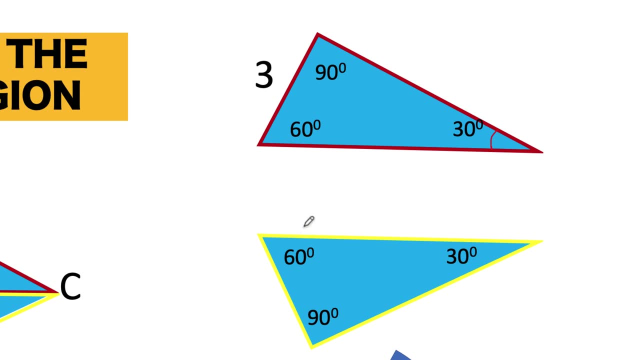 going to subtract the area of this sector. So in a 30,, 60,, 90 triangle the side of this sector is opposite 30 degrees is one half the length of the hypotenuse and the hypotenuse is opposite the 90. 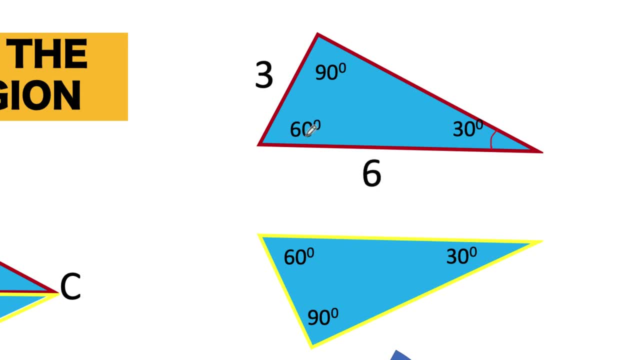 degree angle, And so the measure of the hypotenuse is twice three units or six units, And the remaining side is equal to the measure of the shortest side times square root of three. Knowing these measures, we can now find the area of the triangle. The area is one half times the base. 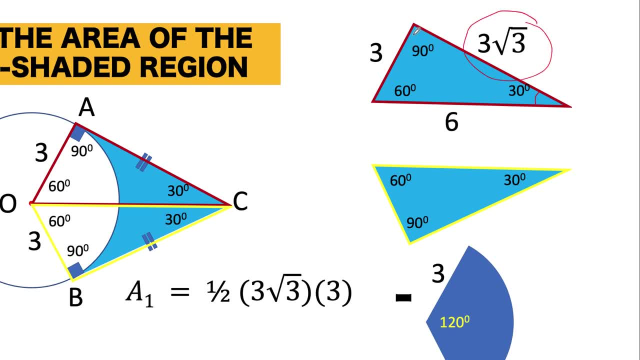 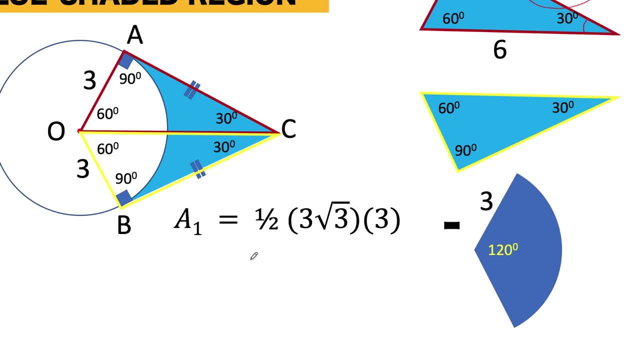 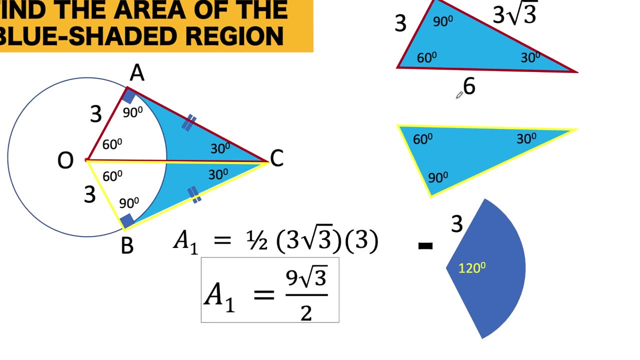 This is our base here, and the height is three units. They are perpendicular with each other. Now, solving for ace of one or the area of the first triangle, this is simplified as nine squared of three over two. Now, since these two triangles are congruent, their areas are also. 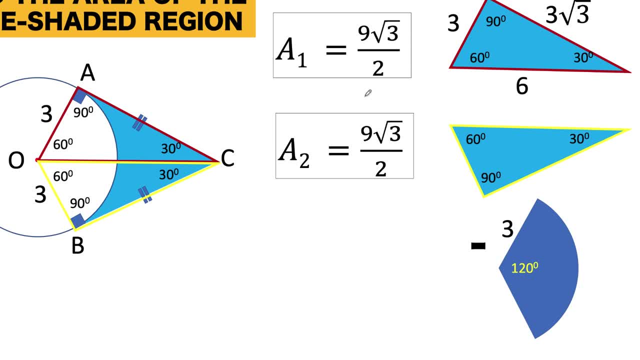 the same. So we need to add these two areas and subtract the area of this sector. So let's find the area of the sector. Let's call it as ace of three. The area of this sector is 120 degrees, over 360 degrees times the area of the circle, with 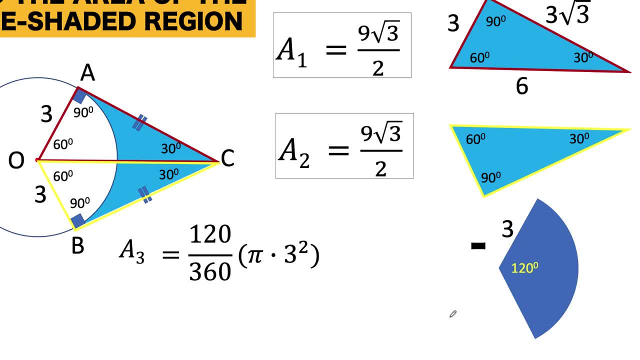 a radius of three units. So pi r squared is the area of the circle with a radius of three units and we get 120 over 360 of that, or one third, And simplifying this resulted to three pi. So the area of this sector is three pi and that is our third area. So we need to add the first two areas. 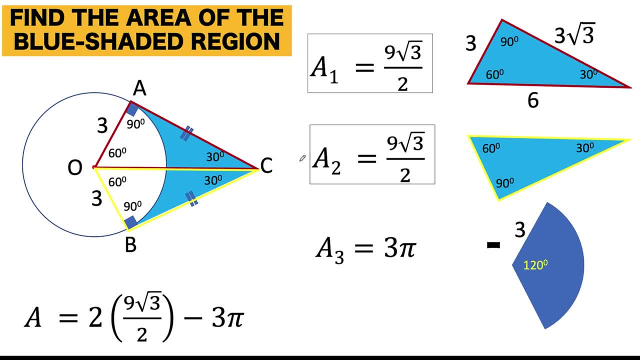 and subtract the third area, So we now have two times this area, nine squared of three over two, minus this area, And this simplifies to nine squared of three minus three pi, And this is approximately equal to 6.16 square units.